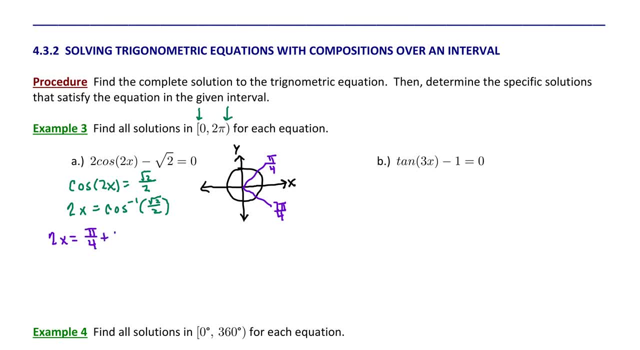 form pi over 4 plus 2k, pi. That expresses pi over 4 and n pi over 4.. So this is the result of any angle coterminal with pi over 4.. In addition, we have 7 pi over 4 plus 2k. 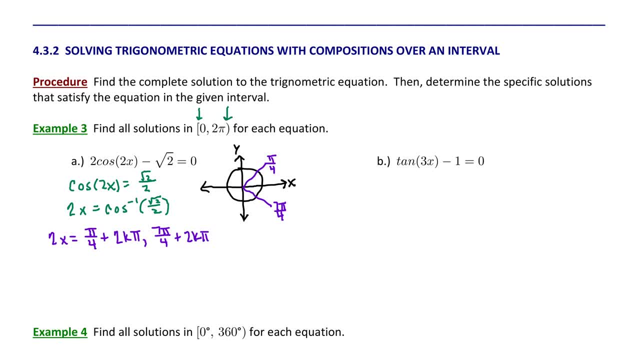 pi. It's at this point that we can go ahead and divide both sides by 2.. Or we can visualize this as multiplying all of the terms in both of these expressions by one half, We'll obtain x equals pi over 8, plus k pi. Again, I'm distributing the one half here And 7. 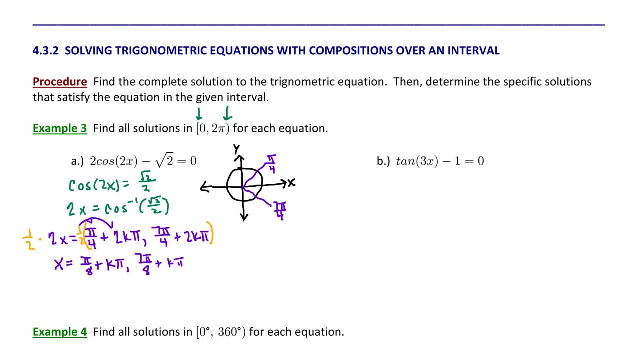 pi over 8 plus k pi, Understanding that k represents any integer. we've expressed every possible solution to this equation in this expression. However, we only want the solutions in one rotation, around the unit circle, So we're going to identify those solutions Clearly. 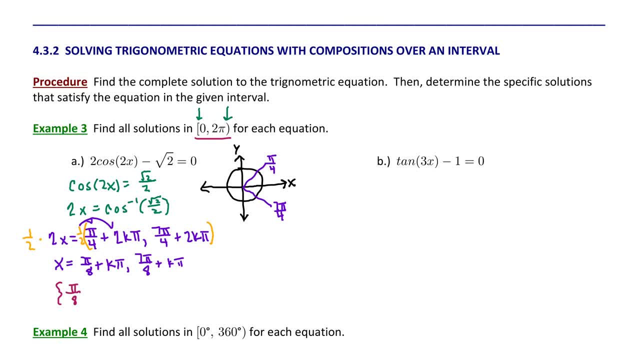 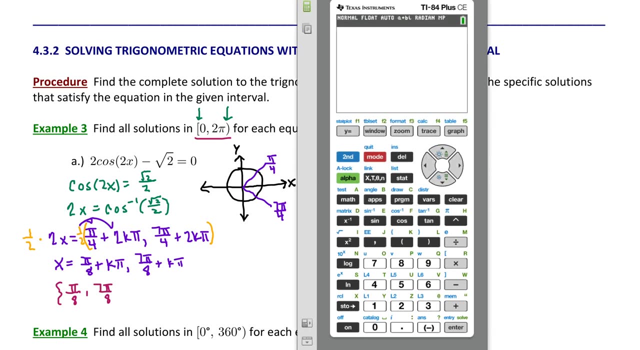 pi over 8 is less than 2 pi and 7 pi over 8 is also a solution. Now we can use our expression, which generates all possible solutions to this equation, to determine if there are more solutions in one rotation around the unit circle. So notice from our first expression: 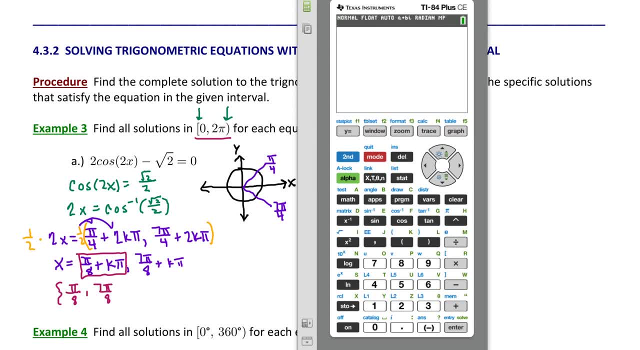 here we have pi over 8 plus k pi. If we allow k to be equal to 1, and I'm going to leave the pi off of my calculation here- if I take 1 eighth plus 1, I'm going to obtain 9 over. 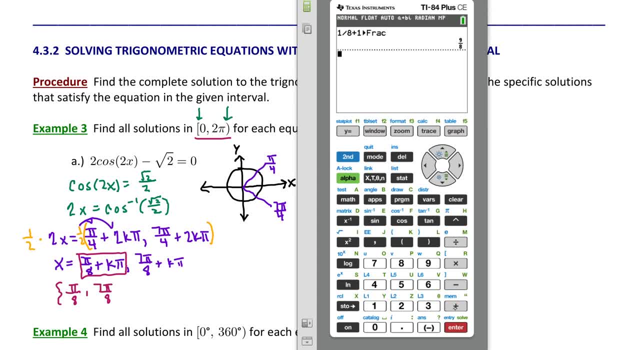 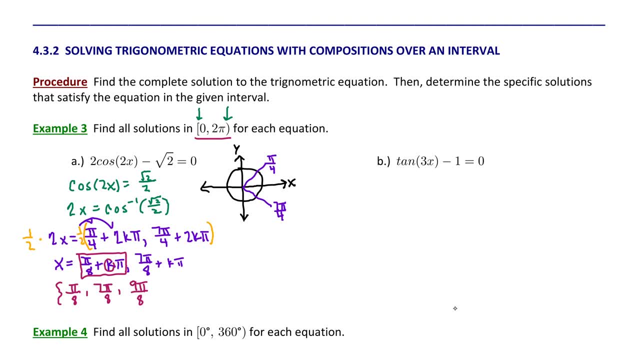 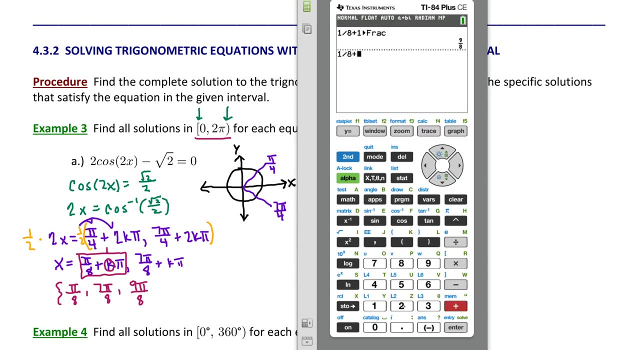 8, or 9 pi over 8.. Now if I substitute in: k equals 2, and I think pi over 8 plus 2 pi, then notice the output is 17 pi over 8.. 16 pi over 8 is 2 pi. so 17 pi over 8 goes beyond one rotation. 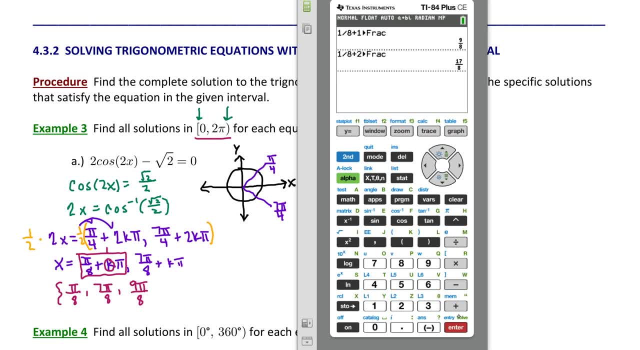 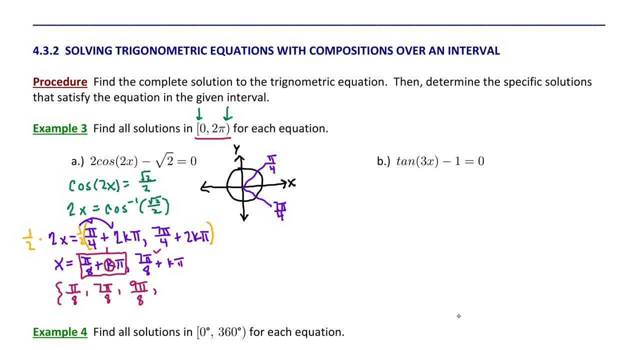 around the unit circle, So we can stop with k equal to 1.. Now let's check out our second solution. We chose the first value- 7 pi over 8, as a solution within one rotation of the unit circle. We can think of that as allowing k to be equal to 0.. If we allow k to be equal, 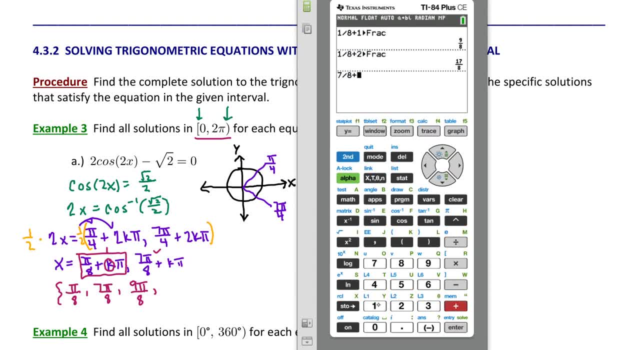 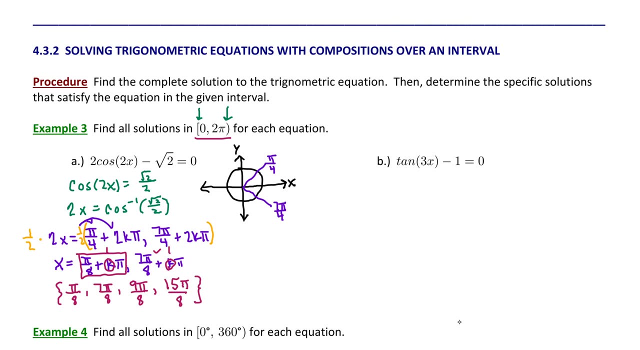 to 1,. 7 over 8 plus 8 over 8 would give us 15 over 8.. 15 pi over 8 is less than 2 pi, so it is also a solution in the unit circle. Again, we just set k equal to 1.. 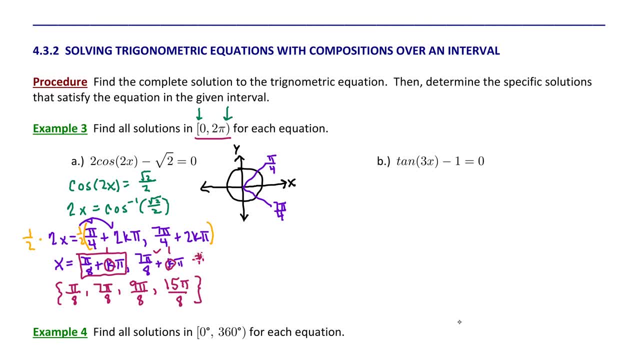 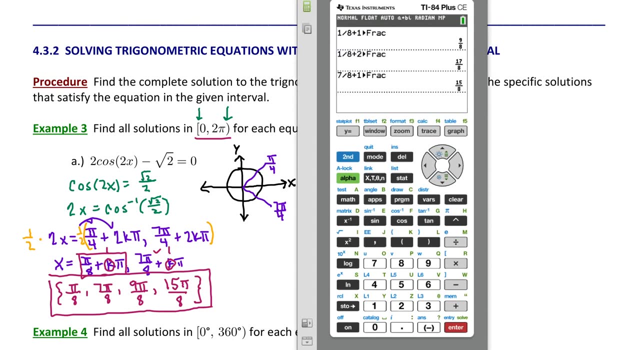 And we use these formulas to generate the individual solutions. So in this case, the equation has four solutions in one rotation around a unit circle. Now it can be easy to overlook solutions, so I always like to verify that I've gotten all of the solutions. 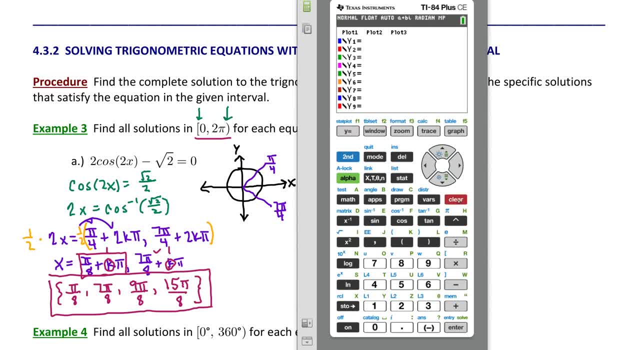 using my calculator. So let's talk about this. I'm going to go to y equals and I'm going to graph the left-hand side of the equation. Notice everything is moved to one side and it's equal to 0.. So if I graph this equation, the x-intercepts will show where the solutions. 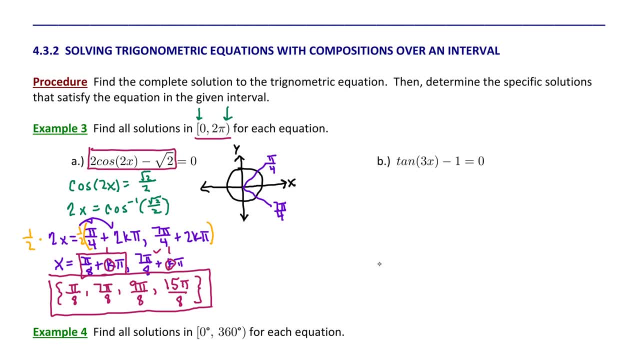 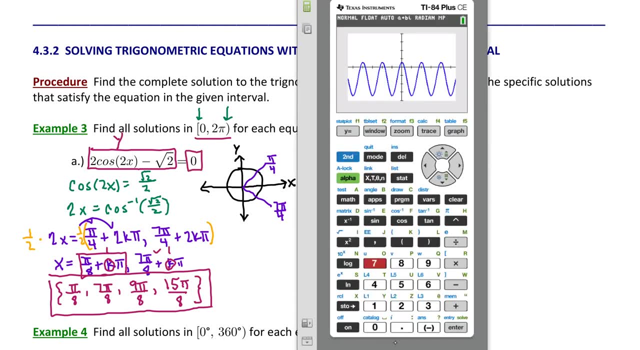 are Because, notice, I'm taking this and I'm letting this be a function y, and we're setting y equal to 0.. If y is equal to 0, we're looking at the x-intercepts. Now I'm going to set: 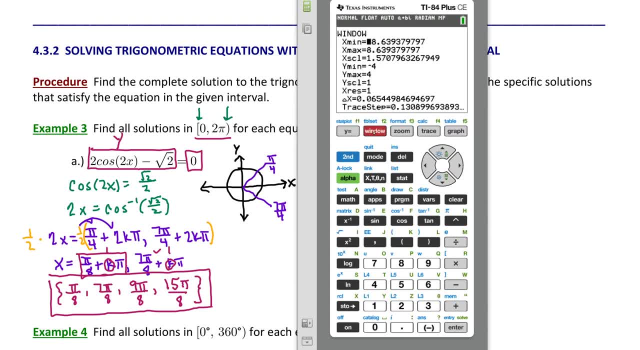 my window very carefully between 0 and 2 pi, and I'm just going to do this manually. So my x-minimum will be 0.. My x-maximum will be 2 pi And, by the way, make sure that you're in radians here Also. 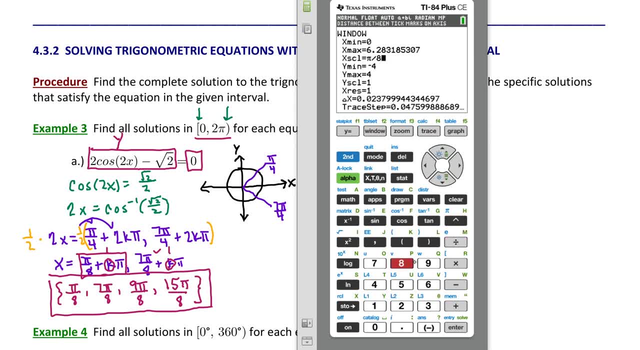 because my solutions are in multiples of pi over 8, I'm going to set my x-scale to be pi over 8, so I can easily recognize my solutions. So notice, in this interval between 0 and 2 pi, we have 1,, 2,, 3, 4 x-intercepts and we came up with 4 solutions, Also because we 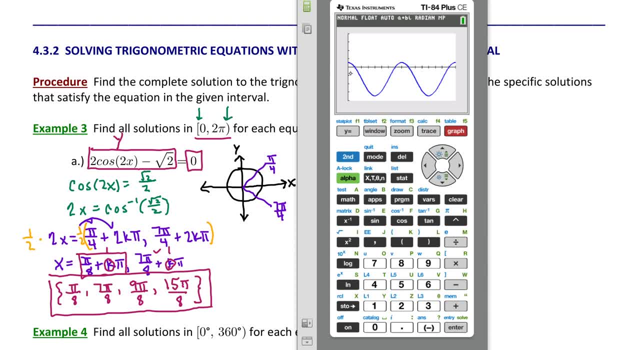 set the scale to be in multiples of pi over 8,. I'm going to set my x-minimum to be 2 pi. We can verify that 1 pi over 8 is the solution, and then I'm going to count 2 pi over 8, 3. 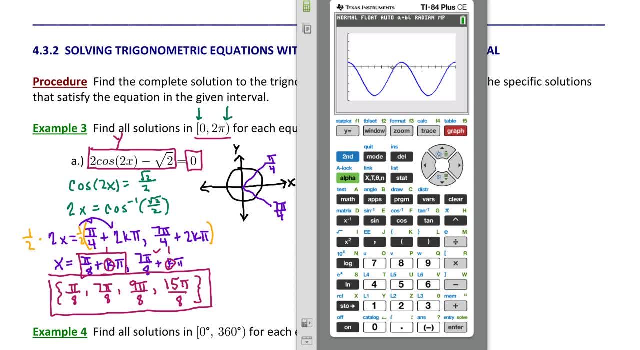 pi over 8,, 4,, 5,, 6,, 7 pi over 8 is an x-intercept: 8, 9 pi over 8,, 10,, 11,, 12,, 13,, 14, and 15. 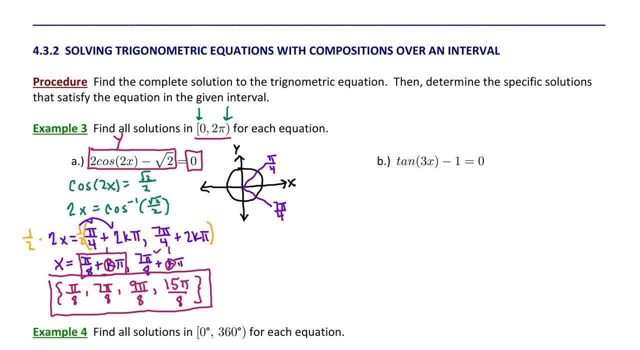 pi over 8 is an x-intercept. So using the calculator, I know for sure. I've covered all of the solutions and I encourage you to use your calculator to double check your work. The whole process of solving this equation is similar to what we learned in the last. 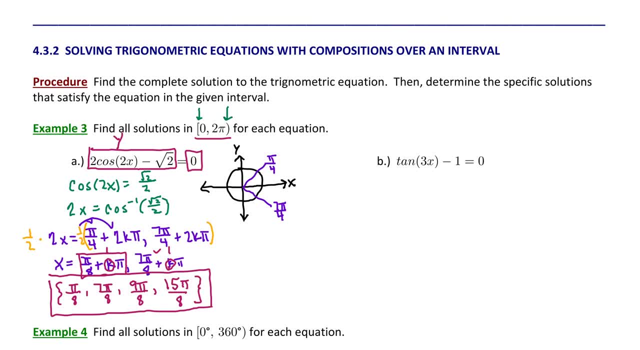 lesson. but now we're getting specific solutions out of our formula. for all solutions, Let's try example B. We have tangent of 3x minus 1 equals 0, so I'm going to isolate the trig function by adding 1 to both sides. We'll isolate the argument by taking inverse tangent. 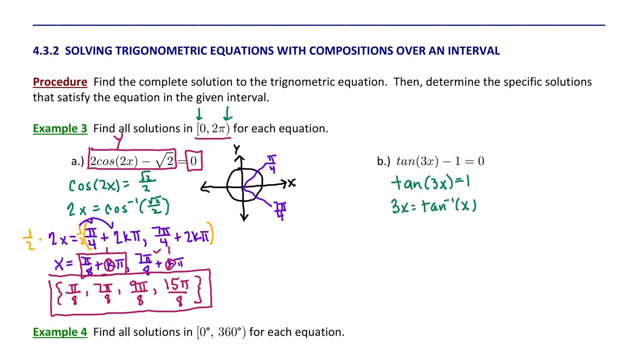 of both sides, but I'm not going to isolate the variable yet. Let's go ahead and look at our unit circle And find all places on the unit circle where tangent is equal to 1.. We know that tangent is 1 at pi over 4, and we also know that tangent is positive 1 at 5 pi over 4.. However, with 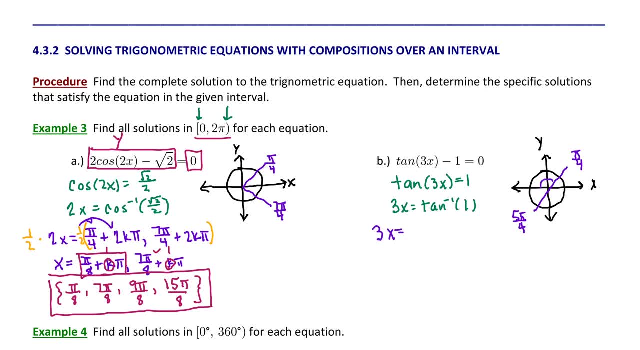 our tangent equations, we recognize that the solutions are pi units apart. so we can express all solutions to this equation as pi over 4 plus k, pi over 4.. Now we can go ahead and isolate the variable. We can see that x equals pi over 12 plus k. 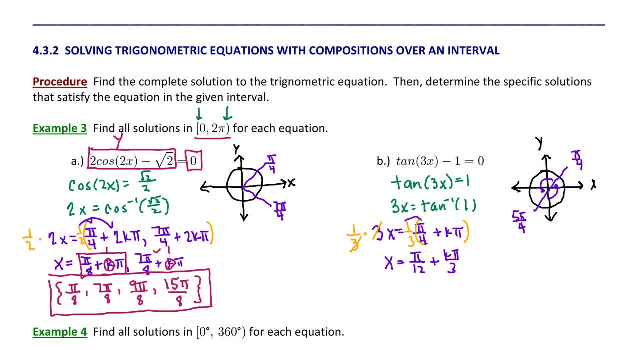 pi over 3.. We're ready to identify solutions that are within one rotation around the unit unit circle That is there between 0 and 2 pi. So if we allow k to be equal to 0, our first solution would be pi over 12 plus 0 or pi over 12.. For my next solution, I'm going to allow k to be 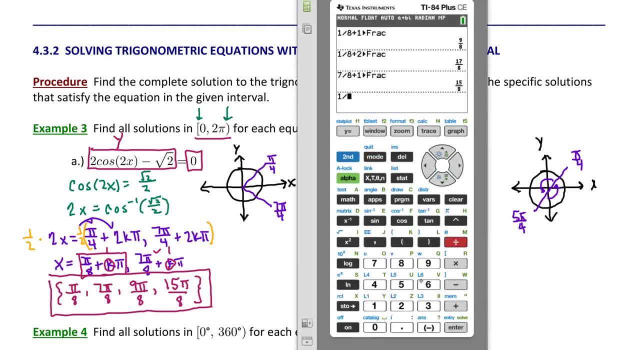 equal to 1.. So I'm going to take pi over 12, and I'm just going to use my calculator plus pi over 3.. Notice, I'm leaving the pi off of my calculation so that the calculator doesn't yield a decimal. 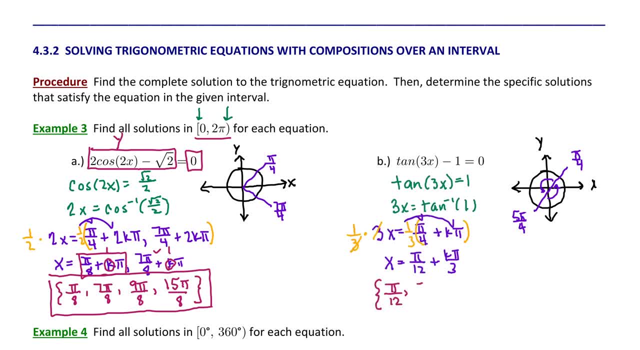 value. So we get 5 12ths or 5 pi over 12, still within one rotation around the unit circle. Next let's allow k to be equal to 2.. So we're going to evaluate pi over 12, or 1 12th plus 2 pi. 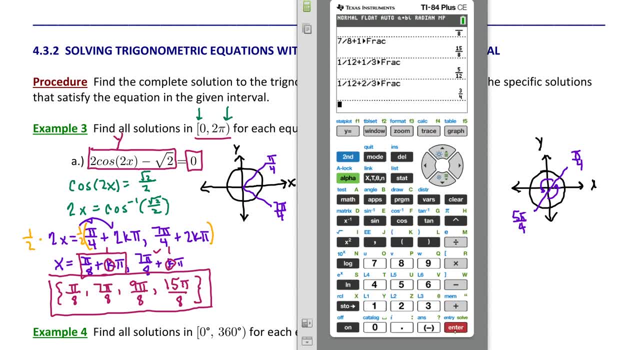 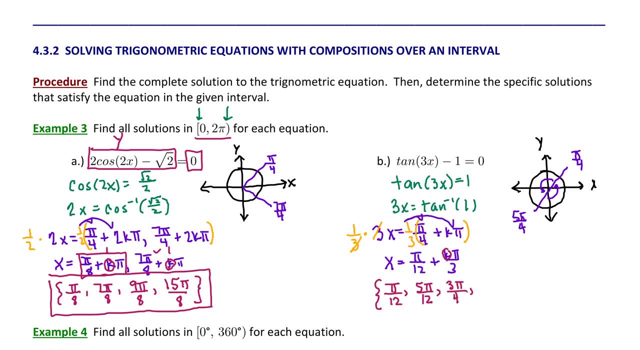 over 3, and I'm going to calculate it as 2 thirds. So we end up with 3 pi over 4.. We're still within 2 pi or 1 rotation around the unit circle. So again, we let k be equal to 0 for the first one, k equal to 1 for the second one, k equal to 2 here. so let's. 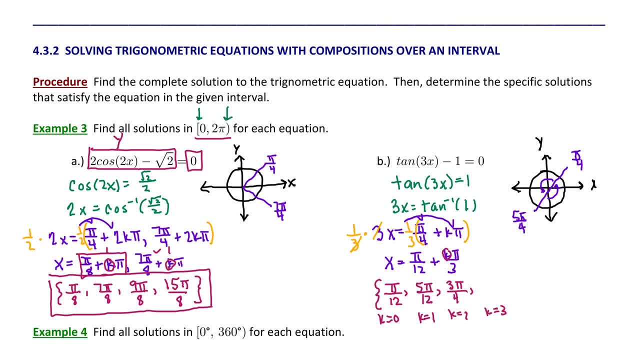 let k be equal to 3.. So we'll take pi over 12 plus 3, pi over 3, or 1 twelfth plus 1.. 1 twelfth plus 12 twelfths is 13 twelfths, or we could say 13 pi over 12.. How do we know when to stop? We stop. 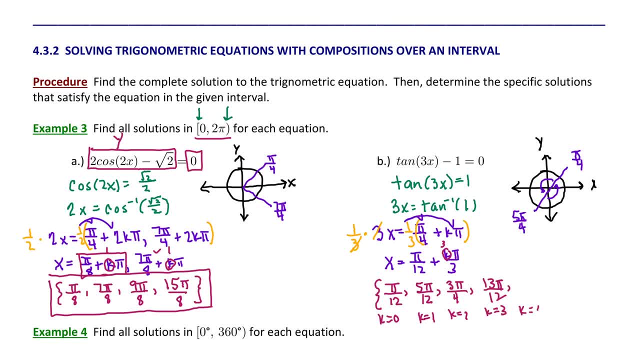 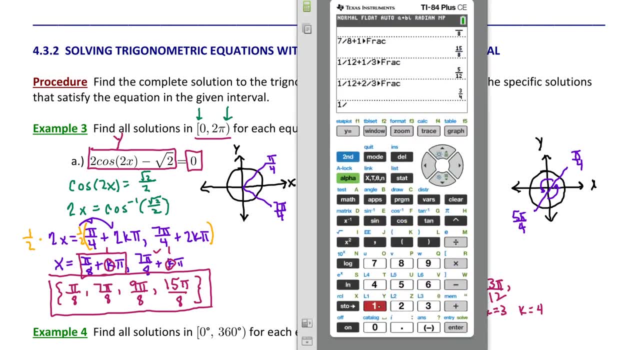 when the value is equal to or greater than 2 pi. So let's update k to be 4.. So we're going to have 1 twelfth plus 4 over 3, representing 4 pi over 3.. I'm just using my calculator for accuracy and 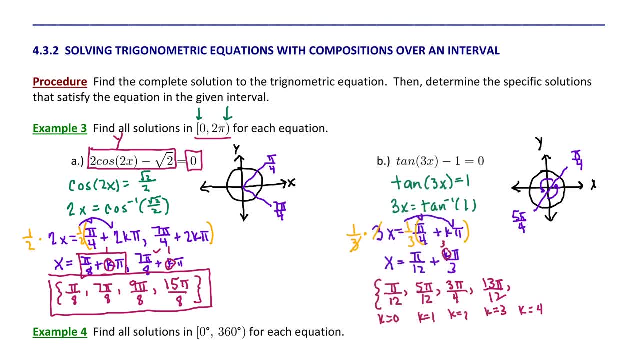 swiftness here and we get 17 pi over 12.. Remember that 24 pi over 12 is 2 pi, so I'm going to keep going until I get either equal to or greater than 2 pi over 12.. So let's update k to be 4.. So let's. 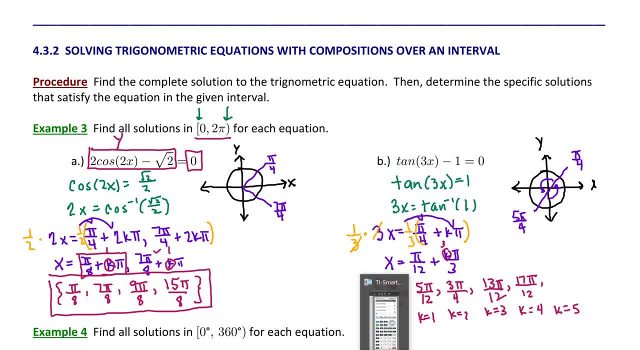 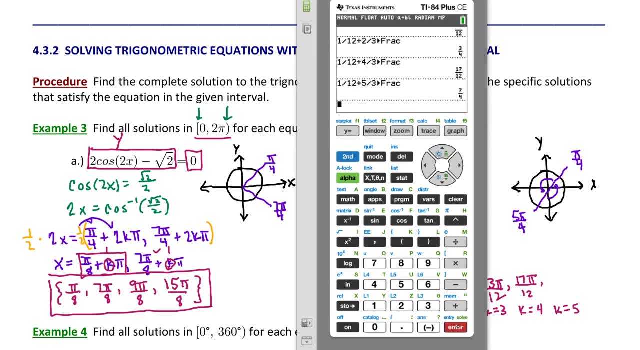 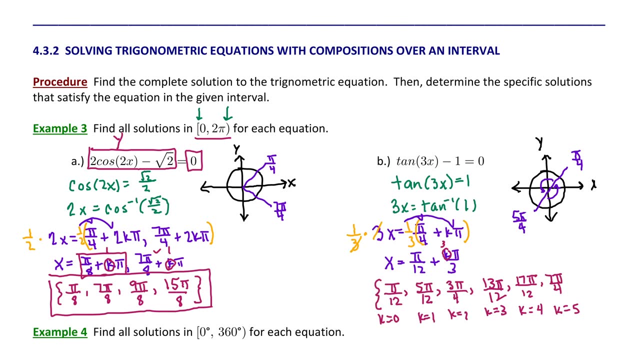 try k equal to 5.. So we're going to have 1 twelfth plus 5 over 3, and that's going to give us 7 pi over 4.. Now if we allow k to be equal to 6,, then we're going to add 6 pi over 3, or 2 pi If I add. 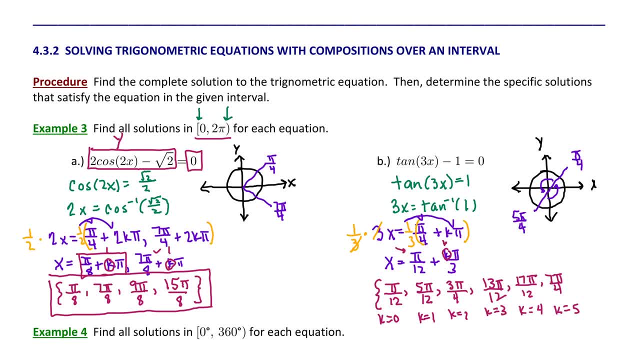 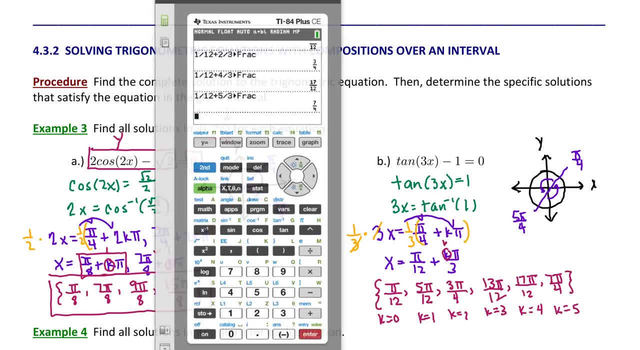 2 pi to pi over 12, then I have gone beyond one rotation around the union. So I'm going to have a unit circle. so we can definitely stop here. We have found 6 solutions in one rotation around the unit circle, but I want to be sure that I've covered all of the solutions, So I'm going to use 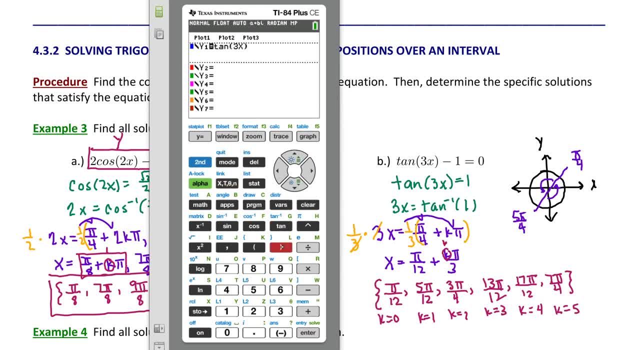 a graph to make sure that I have found every solution in one rotation. So I'm going to graph the left side of the equation tangent of 3x minus 1.. Notice, it's equal to 0 in the original equation. I can translate that into finding x-intercepts of this graph. 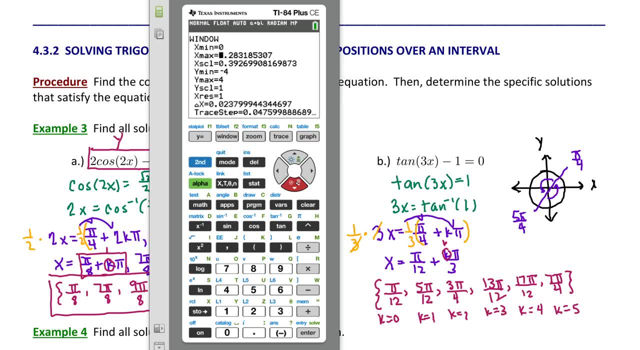 Now we already have our window set from 0 to 2 pi for x-min and x-max. but to make it really easy to recognize my solutions, I'm going to set the x-scale to be multiples of pi over 12, because that's what my solutions look like, And then we can graph the solution. So let's count the x-intercepts. 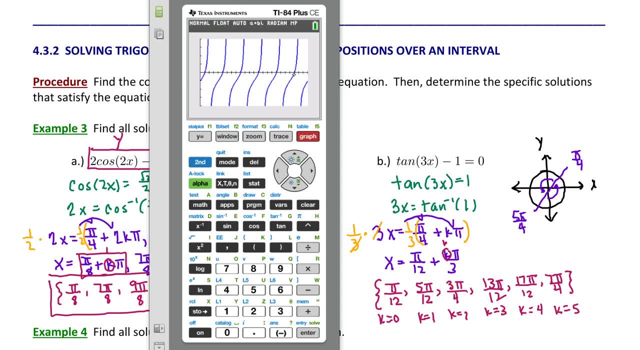 We've got 1,, 2,, 3,, 4,, 5, 6 x-intercepts and we have 6 solutions. So that's a good sign, Also because we've set the scale at pi over 12,. 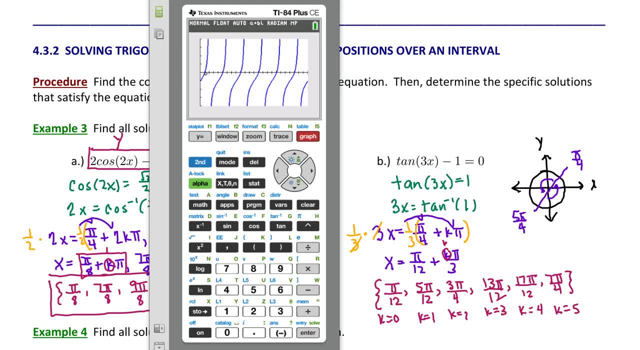 I'm going to count a couple of solutions. The first one clearly crosses at pi over 12,, and then we have 2,, 3, 4.. The next one's at 5 pi over 12,, 6,, 7,, 8,, then 9 pi over 12,. 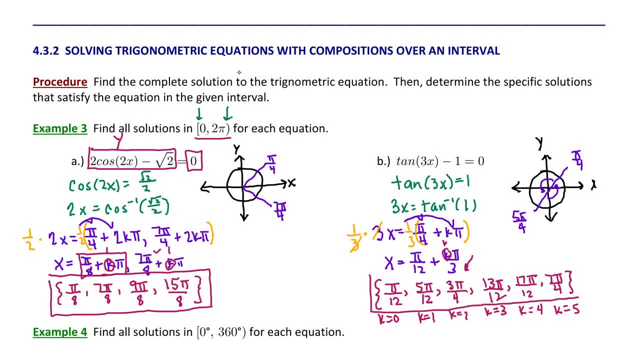 which reduces to 3 pi over 4, so on and so forth. So we can be really confident that we have found all the solutions to that equation in one rotation around the unit circle. These types of equations do require a lot of skill. First of all, we're solving 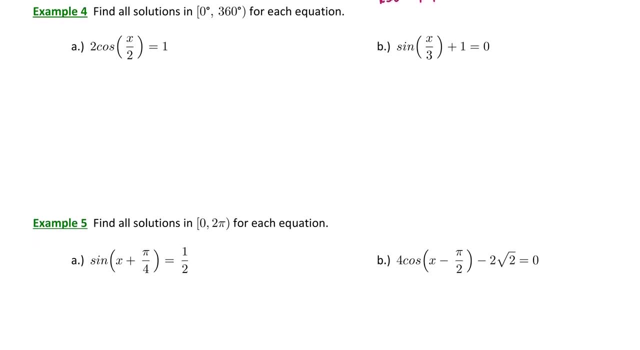 a trigonometric equation. Secondly, we're solving a trigonometric equation with a multiple of the argument or a composition in the argument, and we're not only expressing the complete solution, but we're using that formula to generate solutions within a finite interval. So a lot is going on here and this is going to take some practice. 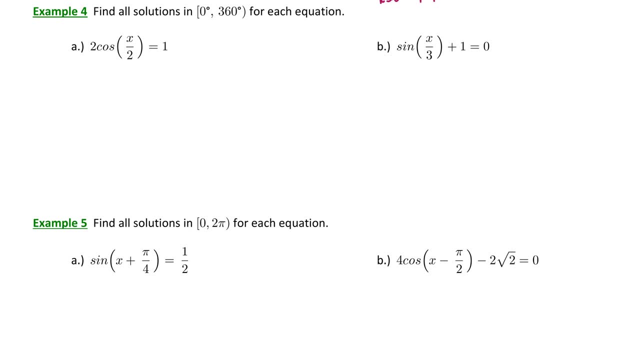 In example 4, I got some good news: We're going to find all solutions in degrees. So again, notice the grouping symbols. If we get 0 degrees first solution, we'll include it in a solution set. but we will not include 360 degrees, because it really 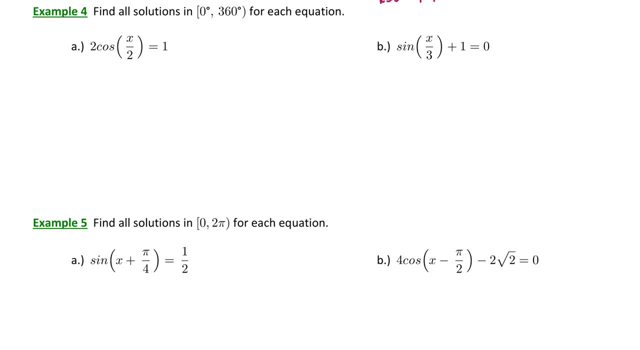 duplicates the solution at zero degrees. 360 and zero are coterminal. So let's solve first for the trig function on example a. We can divide both sides by two. We get cosine of x over two equals one half. Now we're ready to solve for the argument x over two by applying inverse cosine to the other. 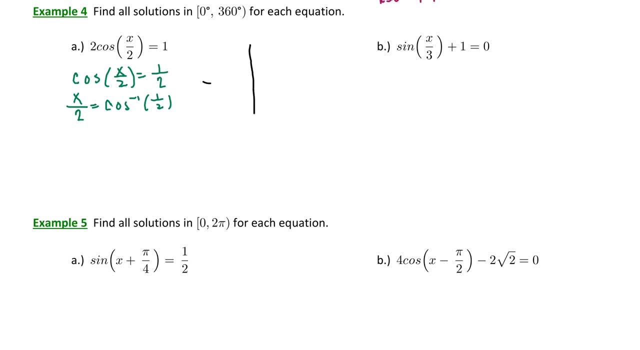 side, Thinking about our good friend and visual tool, the unit circle, I want to find all the angles in one rotation around the unit circle in degrees. with a cosine equal to a half, So clearly that is going to be 60 degrees. Recall that cosine is also positive in quadrant four, so 300 degrees. 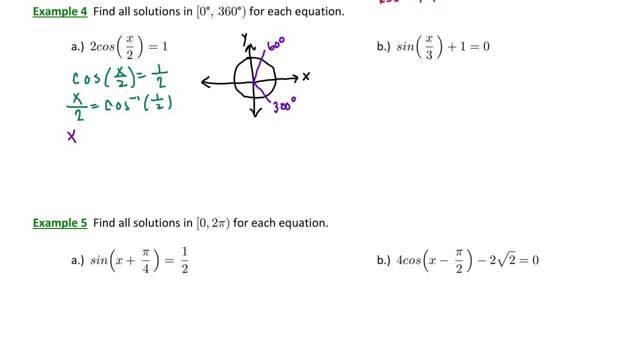 is also a solution. The complete solution can then be expressed as 60 degrees plus 360 degrees times integer k, or 300 degrees plus any angle coterminal with 300. So we'll add again a multiple of 360k. Now that feels good. We got some answers here, but we're 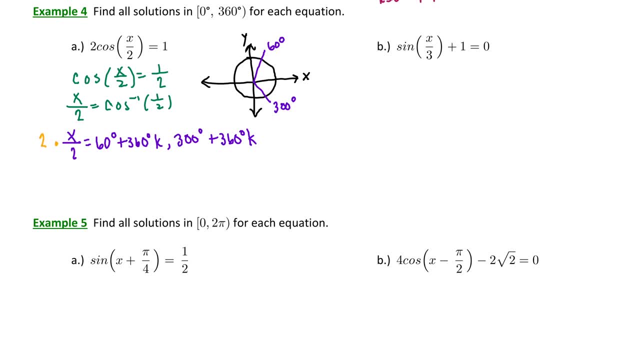 not quite done until we isolate our variable. So I'm going to multiply both sides of all of these expressions by two. Therefore, we have x equals 120 degrees plus 720 degrees times k, or 600 degrees plus 720 degrees times k, where k is an integral. We're getting closer, but we're not quite finished yet. Now 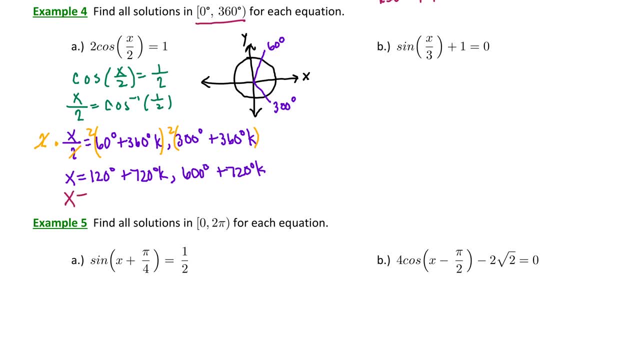 since we're working in a finite integral, we're going to choose only the values that are between zero and 360 degrees. Notice, only one angle is a feasible solution here, and that is 120 degrees. We don't want to add 720 to. 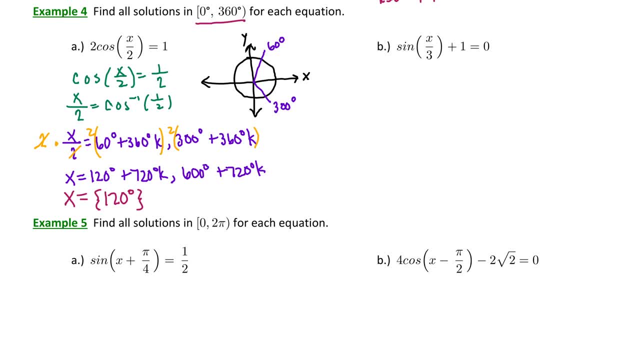 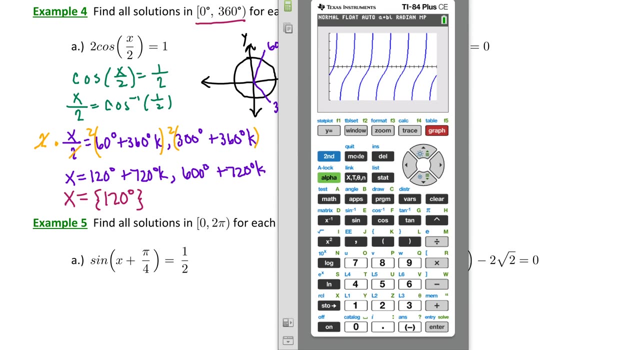 it, because then we'd be beyond 360 degrees and also notice 600 degrees. though it is, a solution to the equation is not in the specified interval, So we only got one solution in this case. To see this on your calculator, we would need to go back to radian mode. So 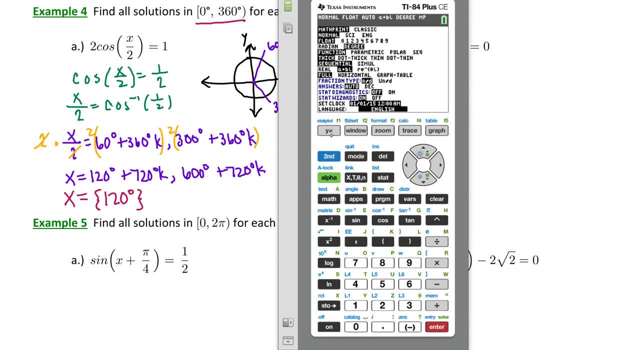 let's- I'm sorry, go to degree mode. We were in radian mode. I'm going to rewrite the equation 2: cosine of x over 2.. Now notice, I want this to be equal to zero, so that I can judge my. 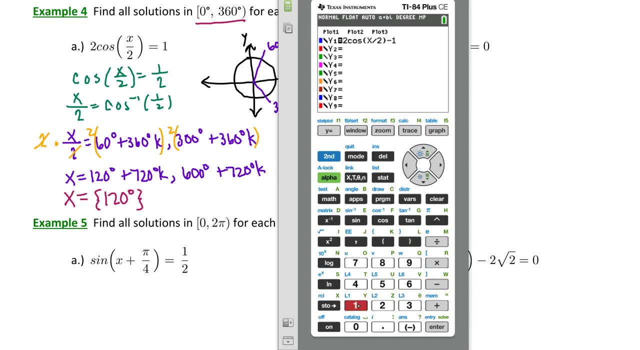 solutions using x-intercepts. So I'm going to subtract the one that was originally on the right side of the equation over to the left side of the equation. Then I can work with x-intercepts Also. let's set our window to go from zero degrees. 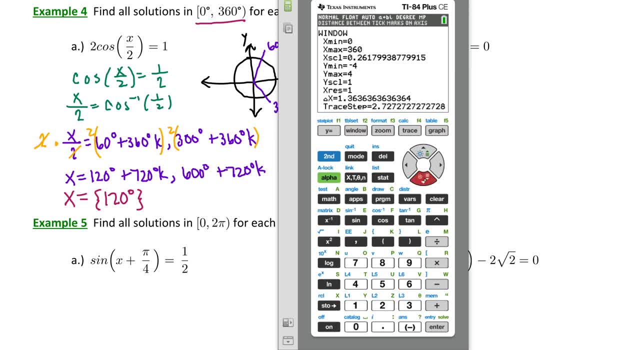 To 360 degrees And you can choose any multiple. I'm just going to go with multiples of 30 degrees for my x-scale And notice we get one solution in this interval, Counting in multiples of 30, we have 30,, 60,, 90,, 120 degrees for the x-intercept, So that really helps. 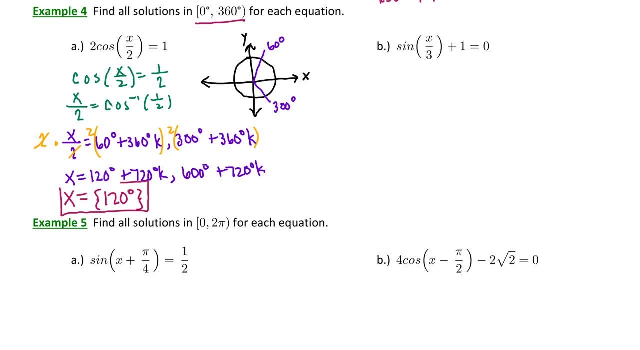 to not only allow us to visualize the solution, but also to verify that we've got all the solutions in that interval. Let's practice that again. So, on example B, the first thing we need to do is isolate our trigonometric function. 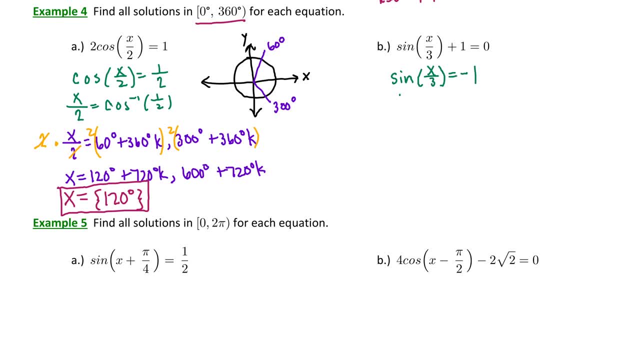 And we do that by subtracting 1 from both sides, Then we're going to solve for the argument by applying inverse sine to the other side, Consulting the unit circle, And you don't have to draw it out. I just find it very helpful to visualize the solutions. 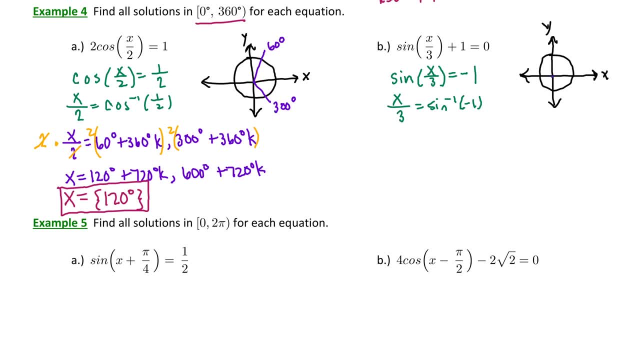 We want to find all the angles on the unit circle with a sine value of negative 1.. And there's only one location. It's 3, pi over 2, or n degrees, 270 degrees. So we can say the solution x over 3 is equal to 270 degrees, plus any multiple of 360 degrees. 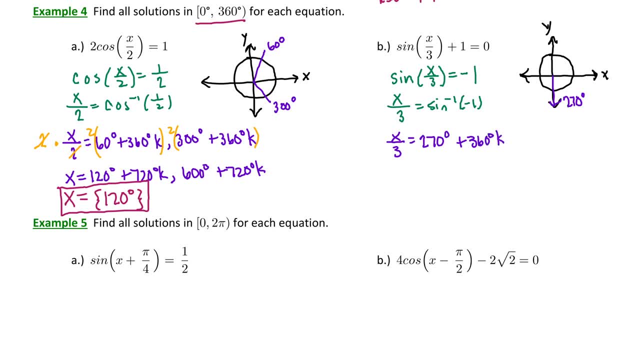 Remember I'm starting by finding the complete solution. Then we are going to solve for the variable x by multiplying all of the parts by 3.. The formula that generates the solutions is then 3 times 270 degrees, which is 810 degrees, And 3 times 360 degrees gives us: 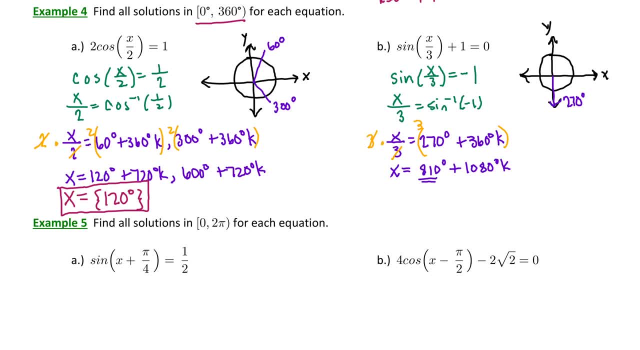 1080k. Notice: even the first solution for k equal to 0 is larger than one rotation around the unit circle. So there are no solutions of this equation that are between 0 and 360 degrees. Now be clear that you understand. this equation does have an infinite number of solutions. 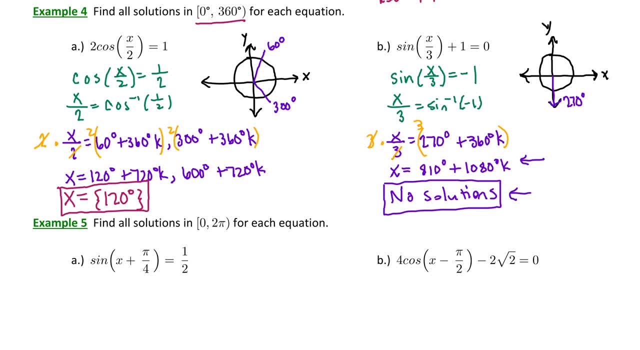 but there are no solutions in one rotation around the unit circle. Now remember this: 270 degrees was the value of x over 3.. When we solved for x, we got 810 degrees. So no solutions of this equation on one rotation around the unit circle. If you were to graph, 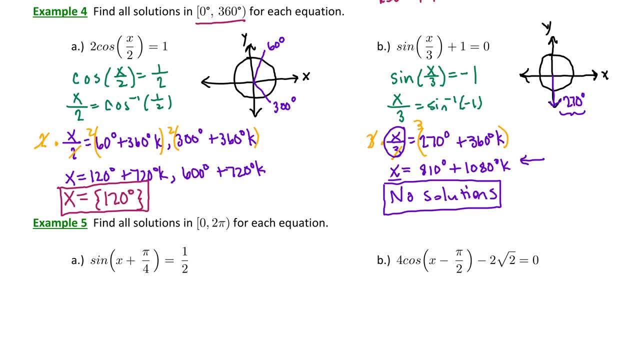 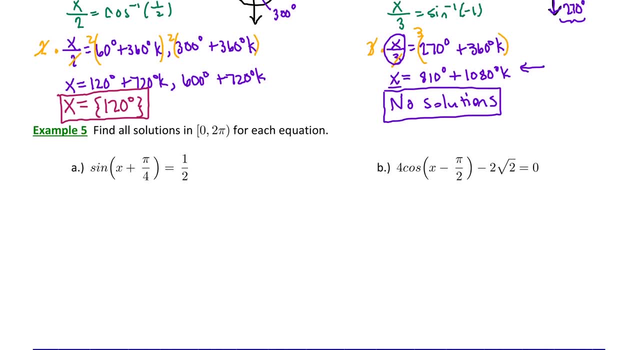 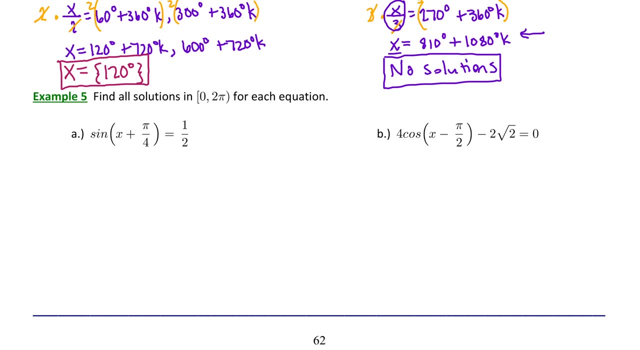 this on your graphing calculator. you would simply observe there are no solutions. You were just going to keep the other solutions. In this lesson we are going to consider one more type of composition. In my opinion, this one is more challenging. In example five we are going to find all solutions in 0 to. 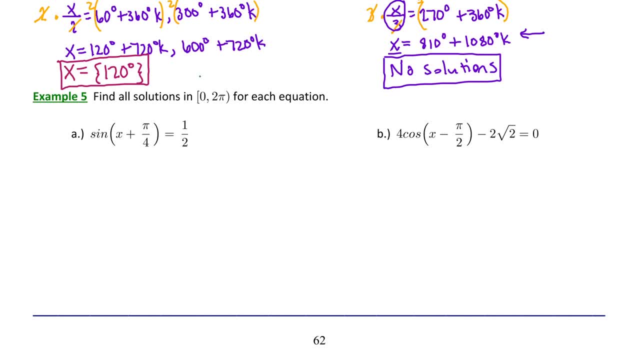 2pi for each equation. So we are back to working in radians Again. notice that the grouping symbols will include zero as the solution, But we are going to stop short of 2pi. What makes these equations different is the argument. Previously, we came up with two equations. 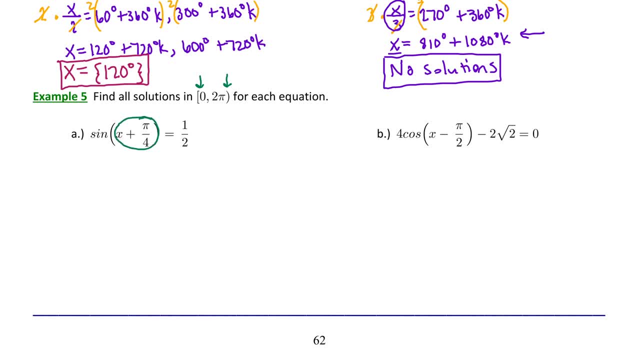 We are going to find 0 to 2pi for each equation, and then we are going to use the argument to find s to match r, And then we are going to add the definitions. What we are going to? we were dealing with a multiple of the argument. Now we have either a sum or a difference in the 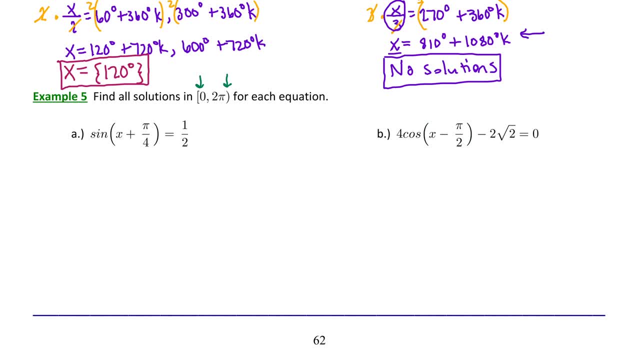 argument. So it's going to change how we handle the very last step, But we're going to start the same way. Number one: isolate the trig function. That's done on example A. Number two: isolate the argument. So we're going to apply inverse sine to both sides and we end up with x plus pi over 4. 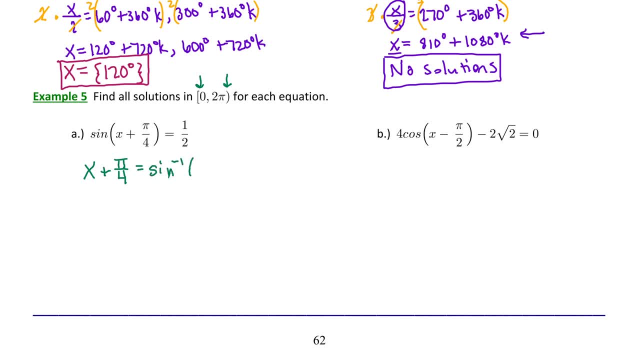 equals inverse sine of 1 half. Now, before I deal with that pi over 4, I'm going to evaluate inverse sine of 1 half, And we'll do that by locating the angles on the unit circle in one rotation which have a sine value or a y-coordinate of 1 half. Observe that sine is equal to 1 half. 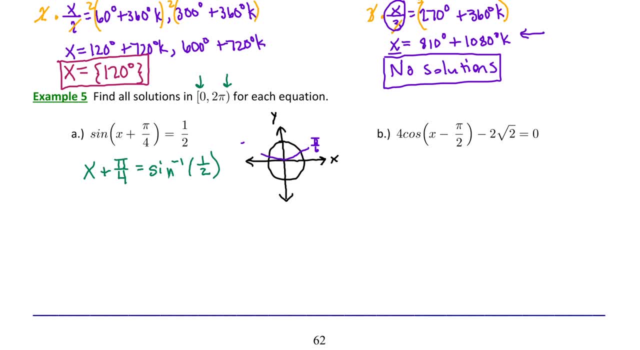 at pi over 6 and 5 pi over 6.. So we can go ahead and express our complete solution for the argument: x plus pi over 4 is pi over 6, plus any angle coterminal with pi over 6.. We express that as adding a multiple of 2 pi, an integer multiple of 2 pi. 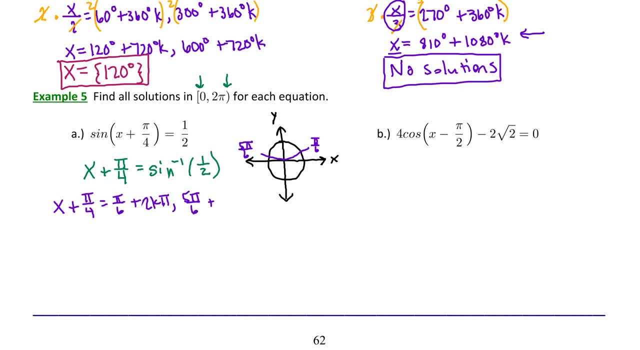 And we'll do something similar with our 5 pi over 6.. Now here's where it gets a little bit different. We are ready to isolate the argument or the variable x, So we're going to do that by subtracting the angle. So we're going to do that by subtracting the angle. So we're going to do. 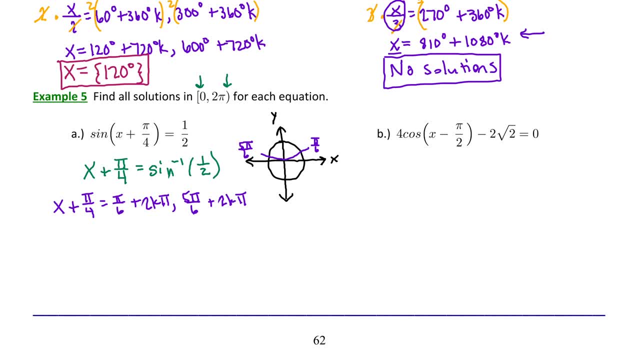 this by subtracting the angle. So we're going to do that by subtracting the angle. So we're going to pi over 4 from both sides. observe, I do have two expressions on the right side to subtract pi over 4 from. so when I subtract pi over 4, I not only have to. 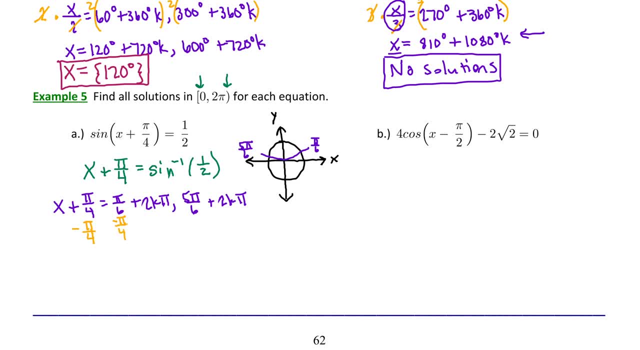 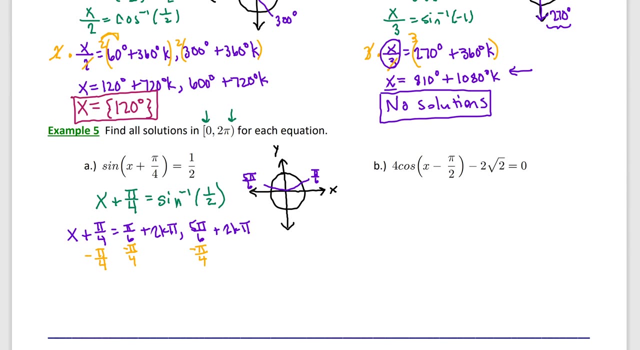 remember to do it to both expressions, but I'm only going to need to combine it with the term that doesn't have the K in it. what's different here? if you glance back up to our previous problem, recall that whenever we multiplied both sides by 2, we had to distribute inside parentheses. we did that with both. 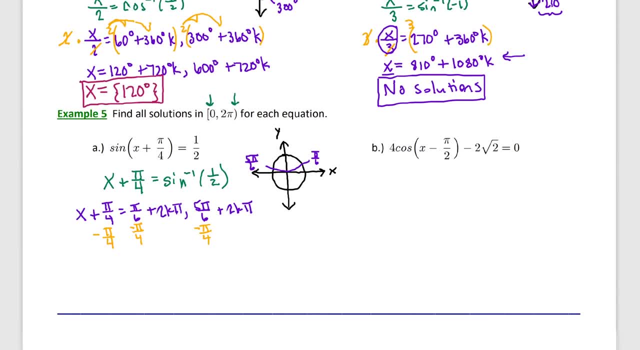 expressions. what's different here is we're not multiplying both sides by something, we're subtracting something, so we're gonna combine like terms. this means I'm only going to combine that pi over 4 with the term without the K. clearly X is isolated on the left side and because my brain is tired, I'm going. 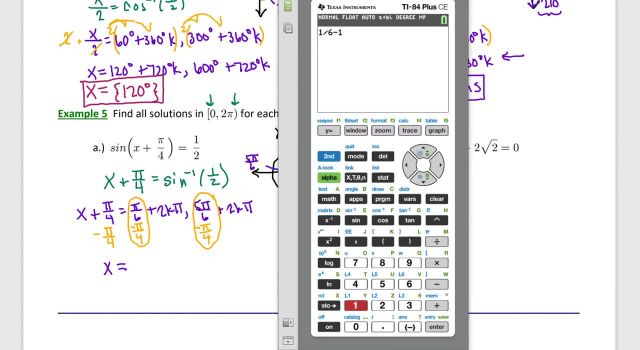 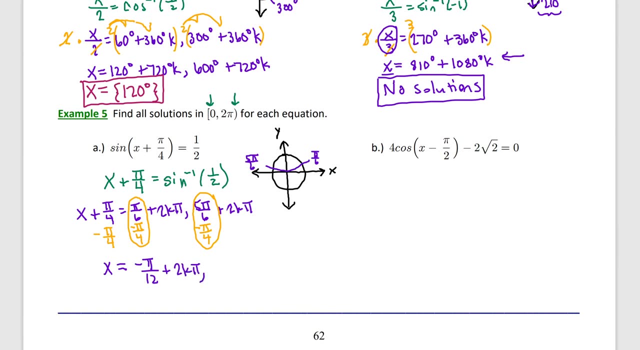 to use my calculator: 1 over 6 minus 1 over 4. I'm using this to evaluate pi over 6 minus pi over 4. we're going to get negative pi over 12 and the 2 K pi stays as is okay. next we're going. 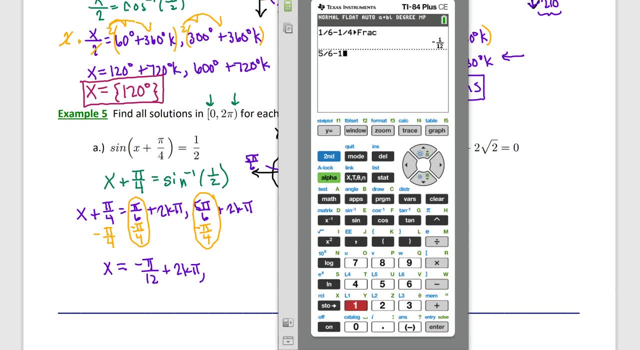 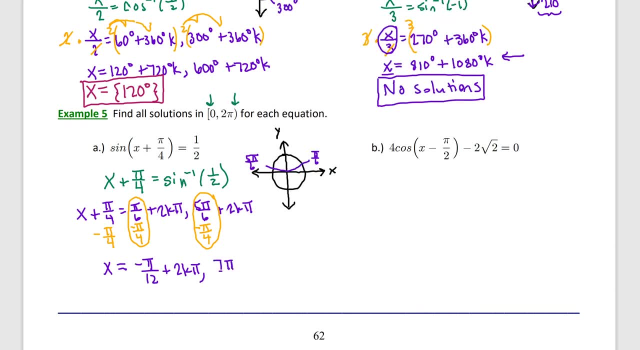 to evaluate 5 pi over 6 minus 1 pi over 4, and I'll do the calculation with the fraction. leave the pi behind and we get 7 pi over 12 and then 2 K pi stays, as is the same. remember that part was altered whenever we had a multiple angle. 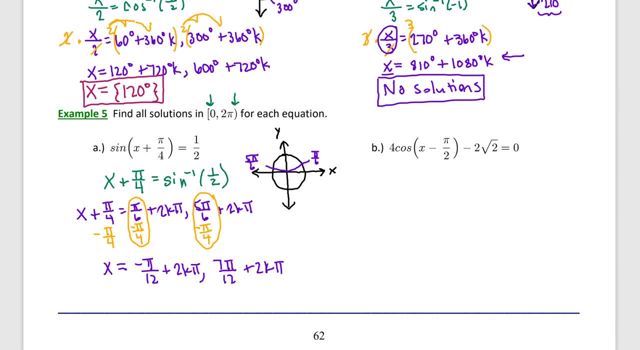 equation. our next step is to identify which of those solutions using this generating formula are between 0 and 2 pi. now notice: negative pi over 12 is less than 0. it's not in the interval, so I'm not going to include negative pi over 12. 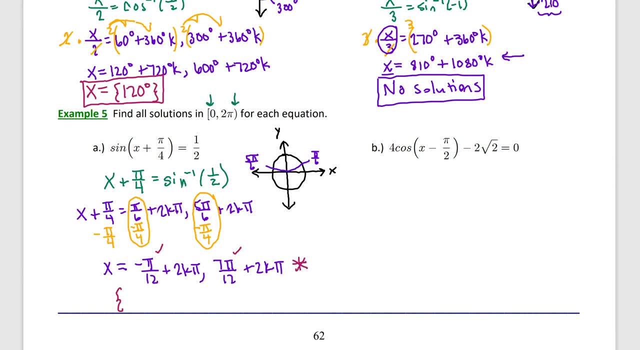 as one of my solutions, however, over 12 is between 0 and 2 pi. So for k equal to 0,, the only solution we're going to obtain is 7 pi over 12.. Now let's go back to our first formula. Let's evaluate negative pi over 12 plus. 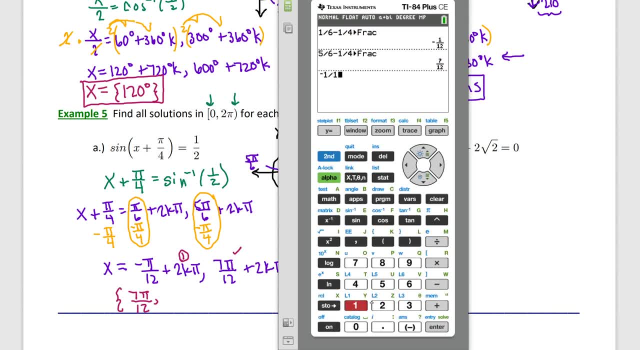 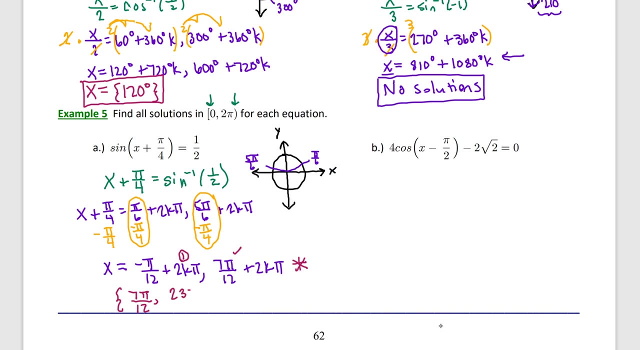 2 pi or negative 1, 12th plus 2.. We're using k equal to 1 here and don't forget k can only be an integer. We obtain the value 23 pi over 12.. Remembering that 24 pi over 12 is 2 pi. 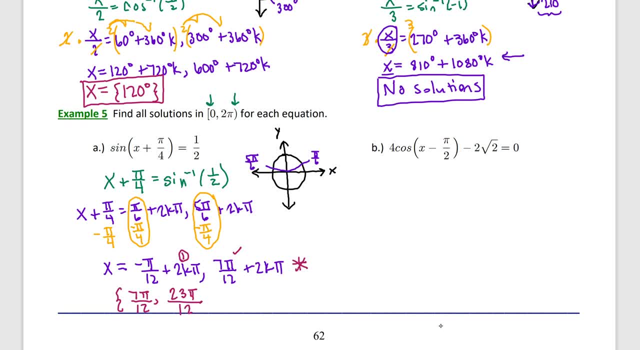 we are really close to the edge here. Now, if we take 7 pi over 12 and we add 2 pi, it's going to be bigger than 2 pi. so it looks like we found our two solutions, But let's be absolutely sure. 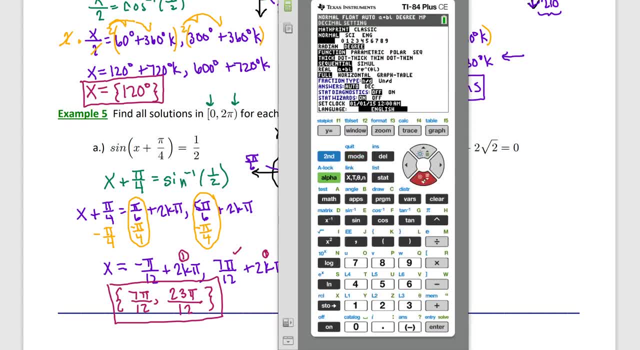 I highly recommend, especially if you're taking a test, to double check your work with the calculator. So I'm going to switch over to radian mode and go to y equals and I'm going to type in, close to the original equation: sine of x plus pi over 4.. But remember, I want to set the function equal to 0. 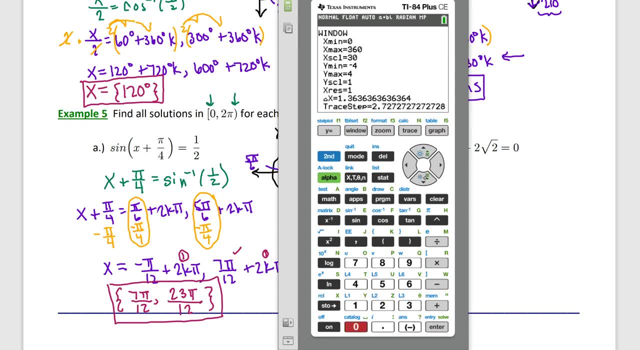 so that I can observe x intercepts as my solutions. Now I'm back to working in radians, so I'm going set my x minimum to be 0 radians, my x maximum to be 2 pi radians. I think a convenient scale to use. 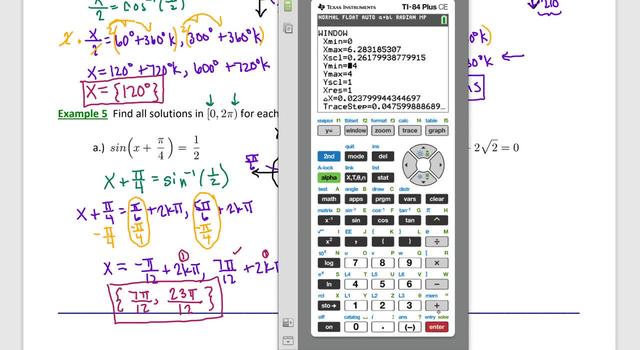 over 12, since both of our solutions are multiples of pi over 12.. So when we graph our function we can observe there are two x-intercepts. We got two solutions And we could carefully count in multiples of pi over 12 to verify the two solutions. 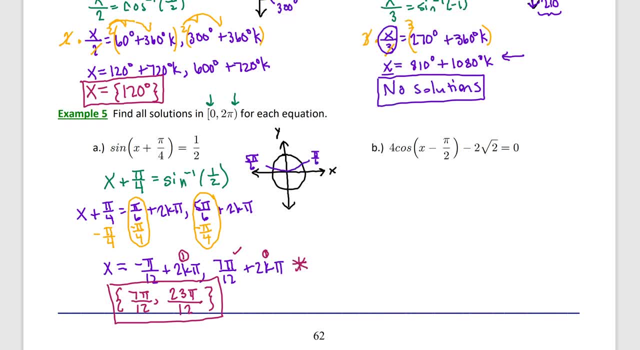 that we obtained. So we did a great job on that one. This is pretty technical stuff, so it's worth it to practice that one more time. On example B, our first step is to isolate our cosine function. So I'm going to add 2 square root of 2 to both sides and I'm going to follow up by 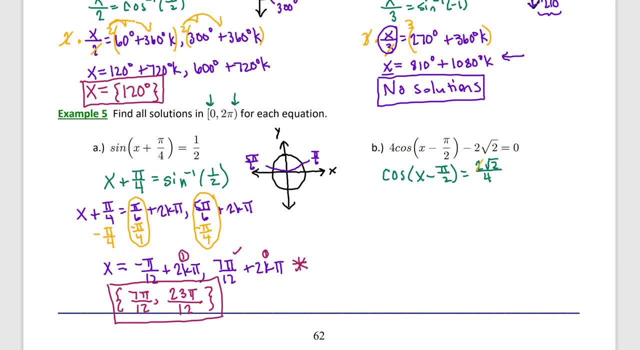 dividing both sides by 4.. This isolates our trig function and we can reduce the right side to see that familiar square root of 2 over 2.. Next we isolate the argument x minus pi over 2 by applying inverse cosine to both sides. 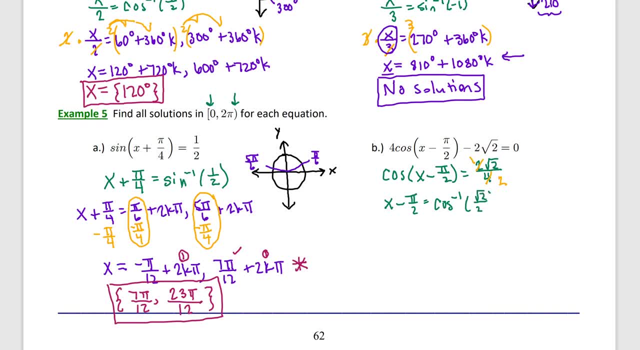 So we need to evaluate inverse cosine, Inverse cosine of square root of 2 over 2 before we deal with that pi over 2 on the left. As always, I'm going to use the unit circle as a visual guide. Helps me to think of where cosine is positive. 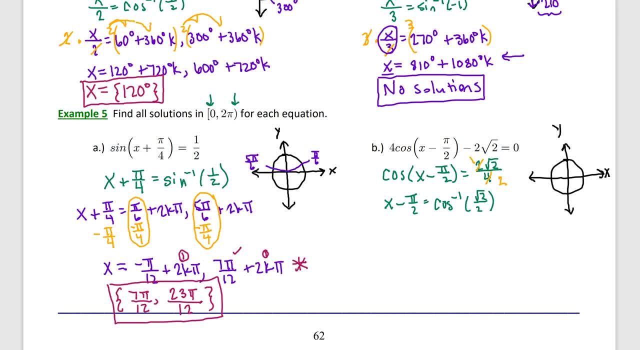 Helps me to think about reference angles. Cosine is equal to positive square root of 2 over 2 in quadrant 1 at the angle pi over 4.. And we also know cosine is positive in quadrant 4.. The value of x is square root of 2.. 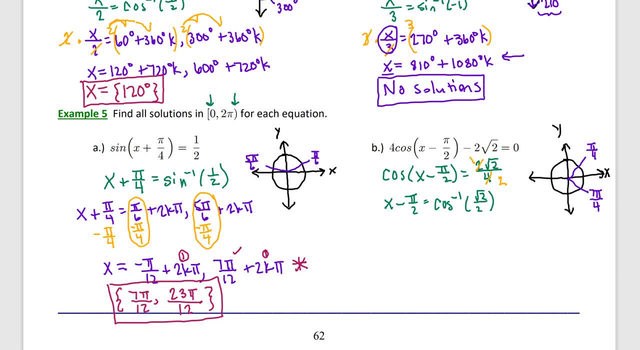 Square root of 2 over 2 at 7 pi over 4.. So it looks like we have two locations in the first rotation of the unit circle where cosine is equal to square root of 2 over 2.. So let's go ahead and express our complete solution. 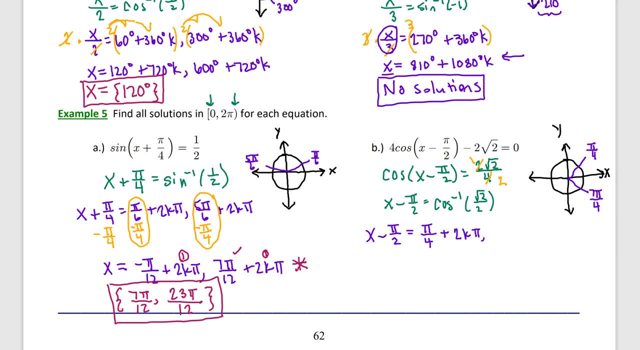 Pi over 4 plus 2k pi and 7 pi over 4 plus 2k pi. K, of course, is an integer. Now we're ready to isolate the variable and we're going to do this by adding pi over 2. 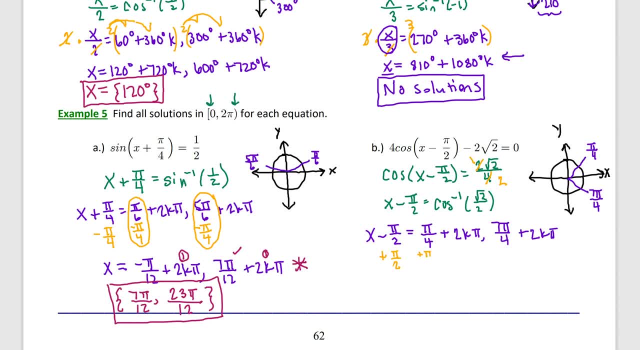 to both sides, including both expressions on the right. Remember you have essentially two equations in 1, separated by this comma here. Also, remember it's only necessary to combine the pi over 2 with the part of the expression that does not have the k. 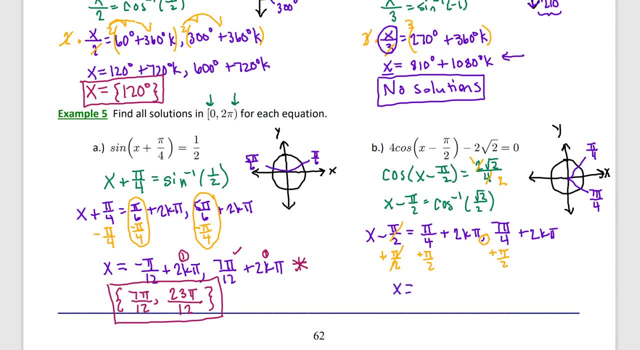 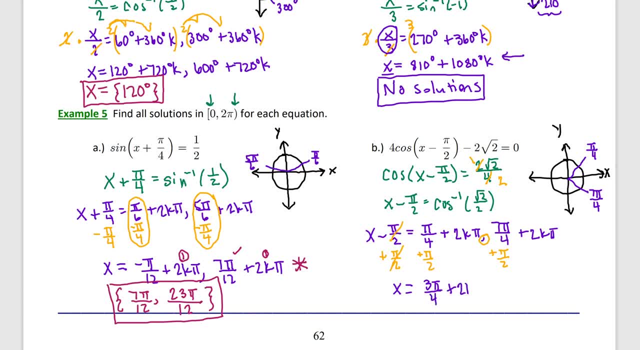 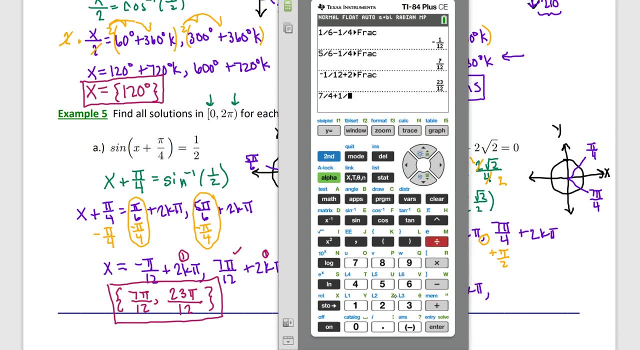 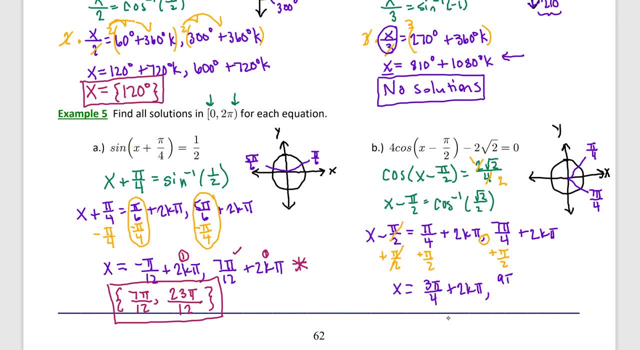 Stick that into the calculator and we get 9 pi over 4.. 9 pi over 4 plus 2k pi. We have gone above and beyond here and found the complete solution to the equation, That is: this is a springboard for generating. 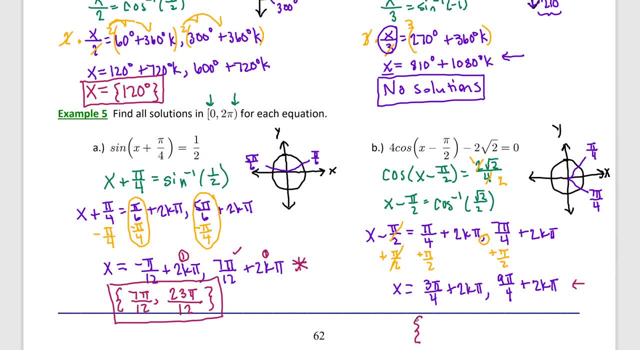 the infinite solutions to that equation for all positive or negative integers, but we only want the solutions within one rotation of the unit 1.. Now we need to recognize, using this springboard or formula for all possible solutions to the equation, Which of these only fits within 0 to 2 pi. 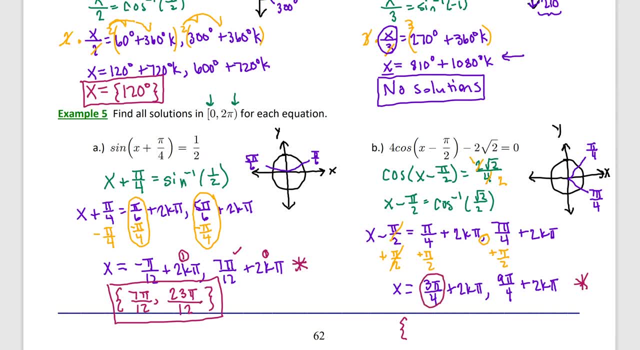 So clearly on this one: 3 pi over 4 is within one rotation around the unit circle. if I add a multiple of 2 pi that's going to cause me to rotate beyond 2 pi. So 3 pi over 4. 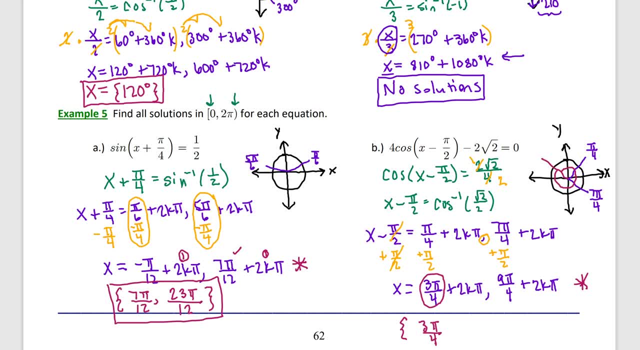 is the only solution that I'm going to get out of that first expression. Now, this one's pretty tricky. Notice the second one: 9 pi over 4, that's bigger than 2 pi. We can think of 2 pi as 8 pi. 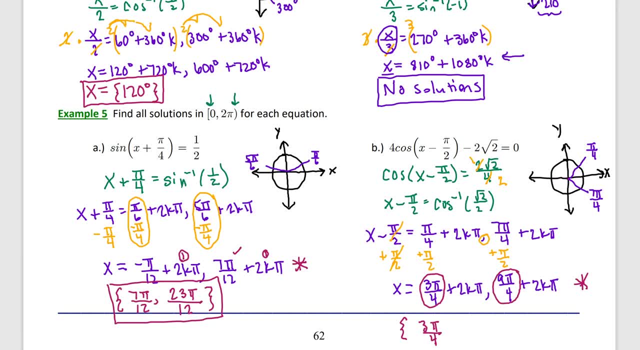 over 4.. 9 pi over 4 is actually coterminal with pi over 4.. So our solution- and let me write these in order, smallest to largest our solutions- will be pi over 4 and 3 pi over 4.. Another way to see: 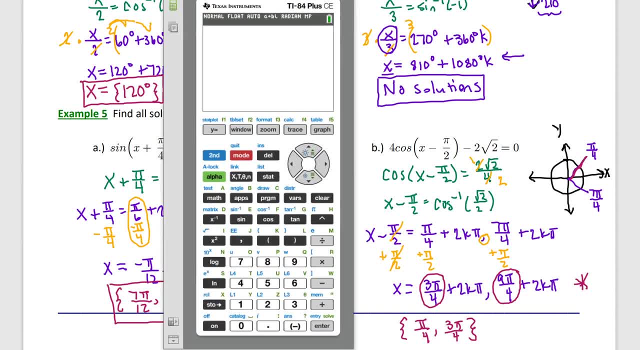 that is to generate it from this second equation. Remember, k is an integer, so it's also possible that k is a negative integer. So if I add 2 pi over 4,, 9 pi over 4 is actually coterminal with pi over 4.. So our solution: 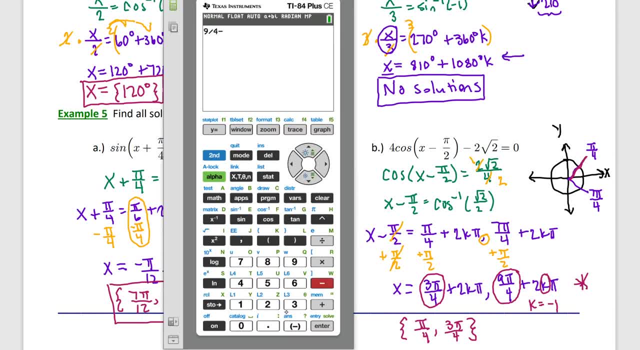 take 9 pi over 4 and I subtract 2, that is minus 2 pi. we end up with pi over 4.. All right, so how do you catch something like that? Well, you may not, but if you check it with your calculator, 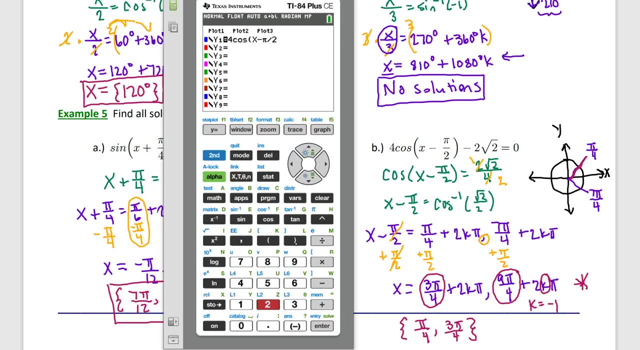 you'll be able to observe, if you've listed all solutions in one rotation around the unit circle And if you have more x-intercepts than solutions, then that would prompt you to go back and look for the other solution. So I'm going to type in the original function Notice: it's equal to 0, so I 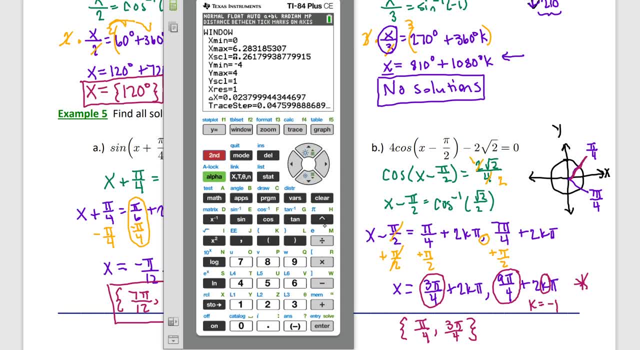 can work with x-intercepts. x minimum is 0,, x maximum is 2 pi, And let's set our scale to be multiples of pi over 4.. So if we take a look at our solution, at our graph, we have 2 x-intercepts. 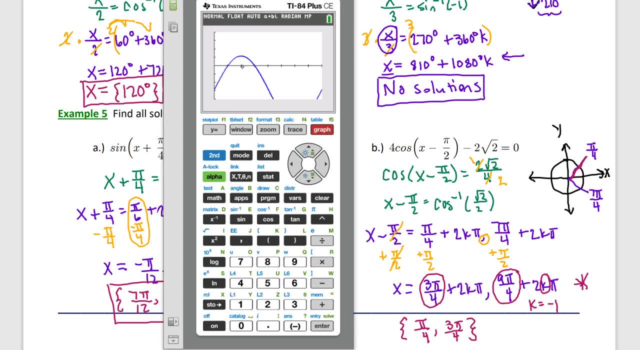 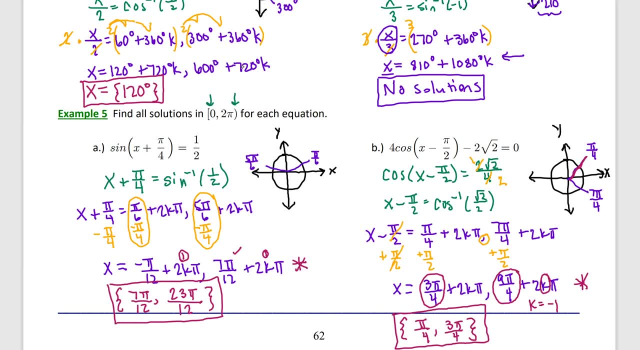 They are located at 1 pi over 4 and 3 pi over 4.. So I strongly encourage you to use your calculator to calculate your solution And I'm going to type in the original function and I'm going to type in double check your work again, this is a really technical section, so if you're